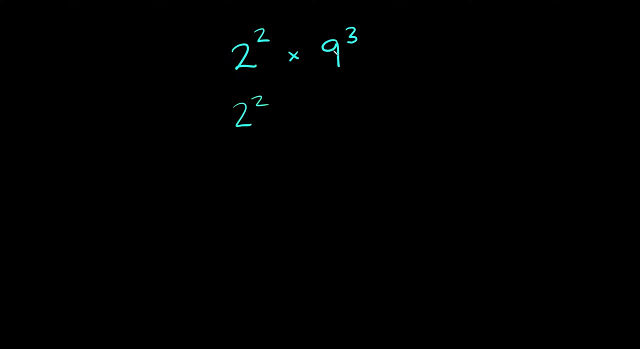 here is: we have two squared right, so we have two squared and then nine right. here we can rewrite as three squared right. three squared is equal to nine, so I'm going to rewrite it as three squared, so we're going to say times three squared, and then we're still raising this whole thing, right? 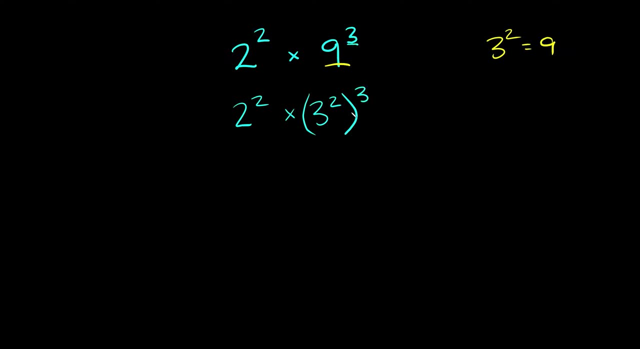 to this third power. Okay, now, one thing I can do here is I can actually flip my exponents here, this two and this three. I can flip them. I can put the three inside and take the two outside. Okay, why can I do that? Well, in order to simplify, an exponent raised to another exponent, we're just 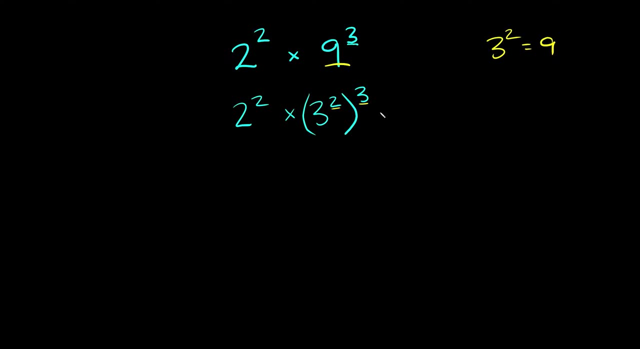 or you just multiply them together, right, and in multiplication order doesn't matter, Okay. so for example here, three squared raised to the third power. well, again, to simplify this, you just multiply them together, right? so two times three is equal to six. so here we really have three to the sixth. 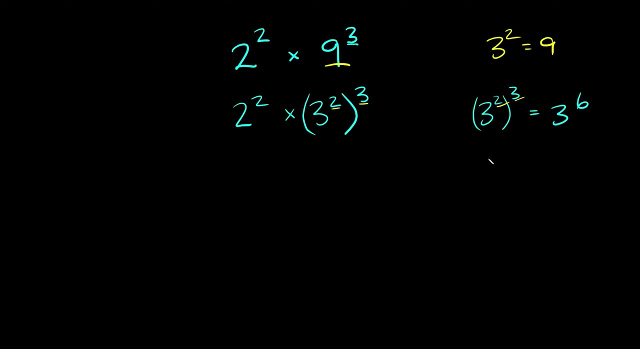 power. Now if I flip them, or if I switch positions here and I wrote it as three raised to the third power right and then put the two on the outside, well again, what's three times two, Six right. so this is still equal to three to the sixth power. Okay, so it's really. 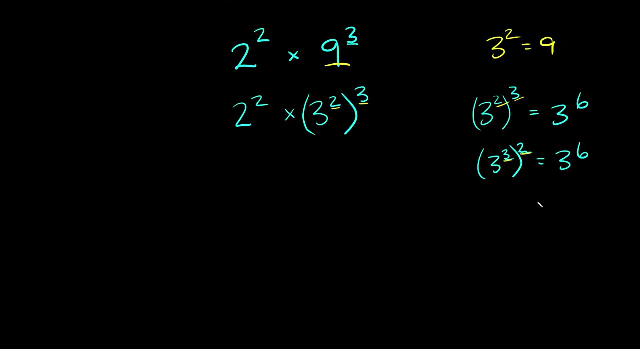 important to know that you can flip your exponents. if it's helpful, Okay, and in this case it's going to be helpful, because if we simplify this a little bit more, so we're going to have two squared times and then again we're going to flip these two, three raised to the cubed or third power. 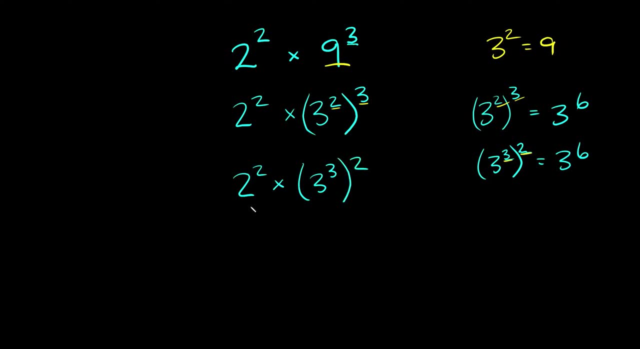 raised to the second power. Okay, so now, as you can see, here we have different bases. right here we have a two, here we have a three cubed. but now we have the same exponents. right, we have a two here and a two here. Okay, so now that we have the same exponents, now this is a little bit easier, Okay. 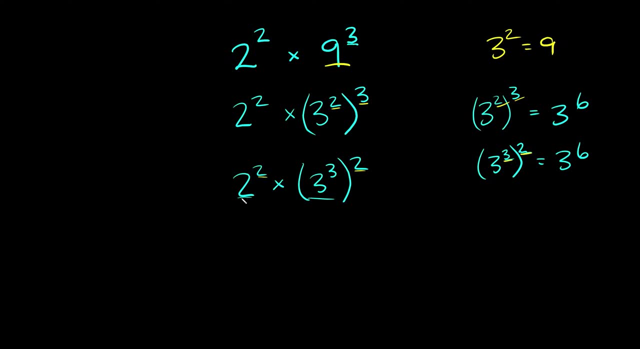 the way you simplify this is: you take your two bases, right? they're different in this case. right, we have a two and a three cubed. we're going to multiply those together, so we're going to say two times three cubed, and then, since this has a two, we're going to multiply those together, so we're. 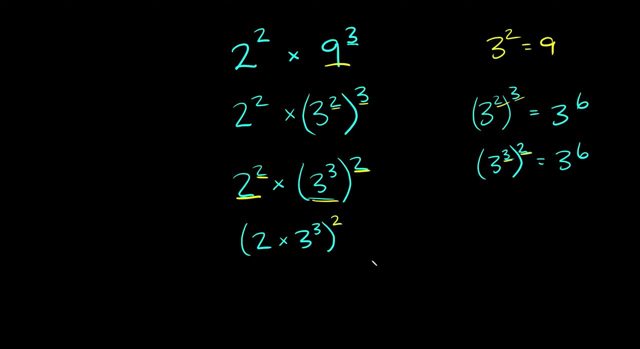 going to say two and this has a two. you raise this whole thing to a two. Okay now, three cubed. we can simplify this a little bit more, right? three cubed is equal to 27.. So inside these parentheses, we really have two times 27, and we still have our exponent out here, right the squared. Okay, so then.